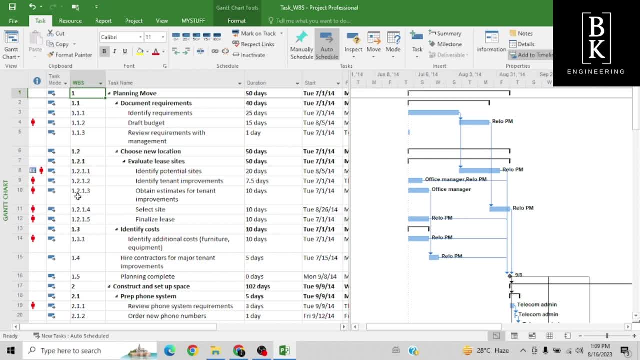 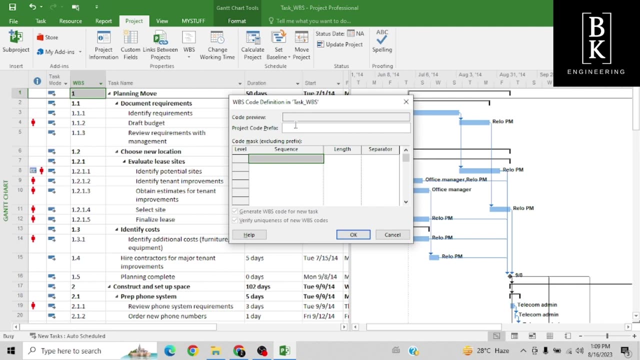 If you are not okay and you want to give a specific numbers, let's give the customized WBS code. Go to the project tab. Here WBS define code. Here we have to give the project code, Prefix anything which you want Here in sequence: first work: There will be a four options number, upper case. 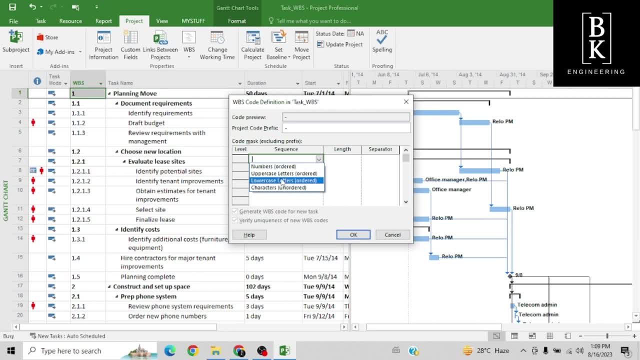 First case means like upper case, A to Z. Lower case means lower letters, A to Z. Characters, like unordered and numbers are in order. First we will go with the upper case letter and second, lower case and third number. Fourth, we will choose as characters. 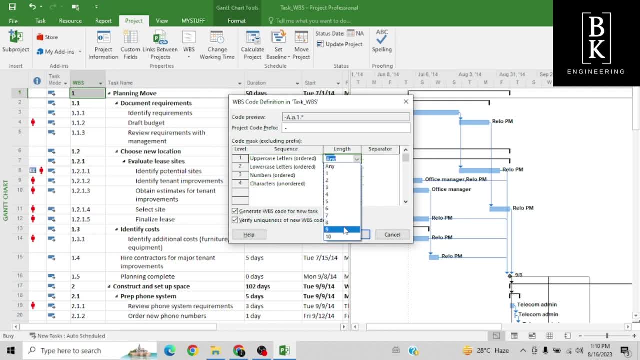 Here we will give any number up to 10.. 1. Here we will give 2. Here let's give again. 1. Say character, 2. Then click OK. See the code preview will be like upper case letter, then lower case letter, number and character. 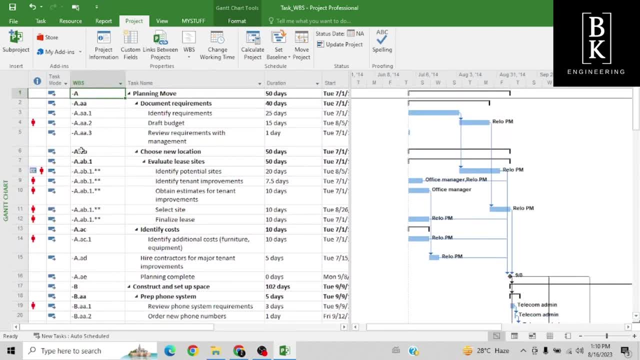 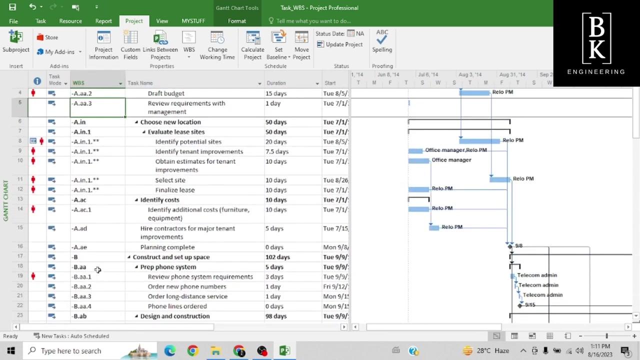 This is the code. If you want to give any specification here, then we can add. Here. we can make anything. See, automatically it has been changed as IN. This is how we created WBS codes. 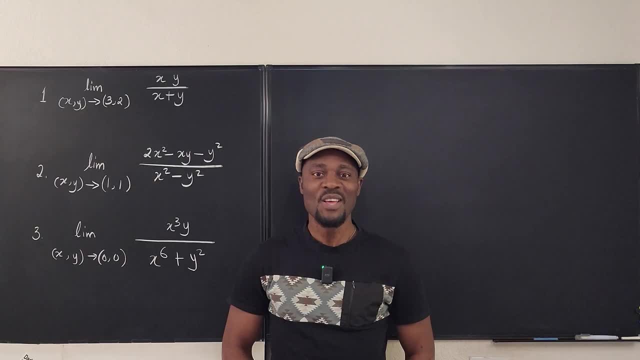 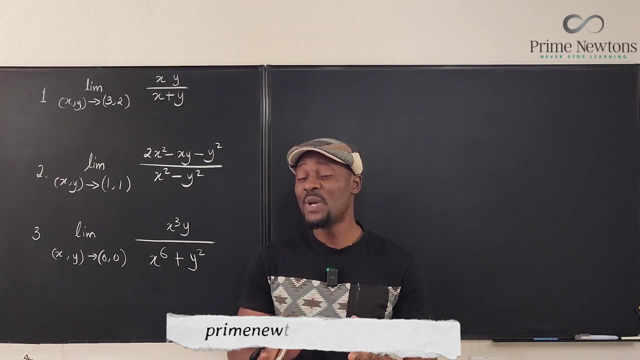 Welcome to another video. Let's take some limits of multivariable functions. We're going to be doing the same thing we usually would do if it was a single variable function, as you did in calculus 1 and in calculus 2.. But you just have more than one variable now and there's nothing.